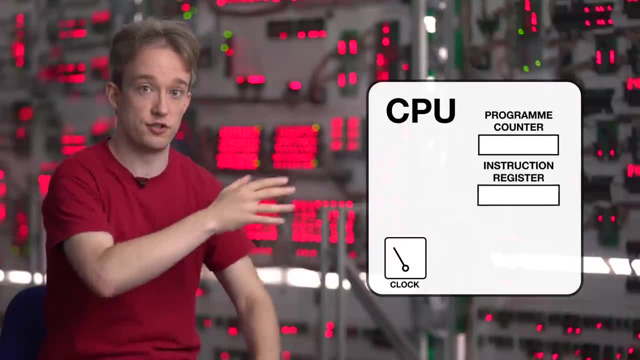 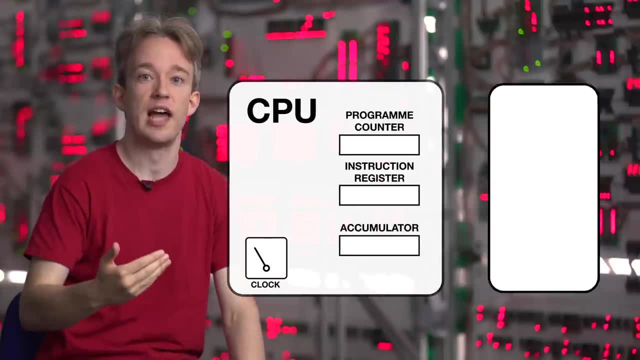 These are a register that keeps track of our instruction cycle, another that loads our instructions from memory and an accumulator. The final thing we need in our simplified computer is somewhere to keep the instructions and any values that we end up calculating. That is RAM, random access memory, and we call it random access because it doesn't matter. 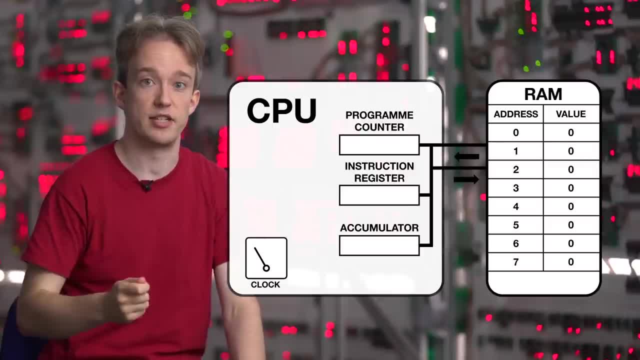 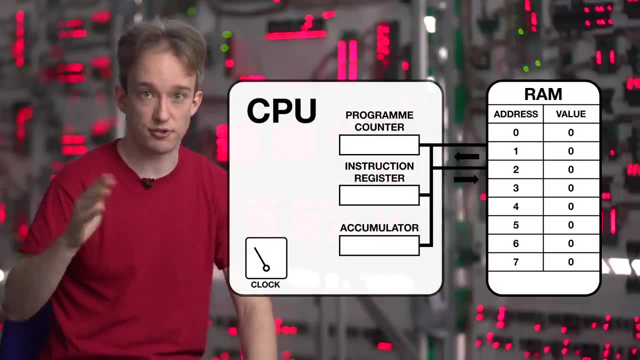 when or in what order the information is read or written. So that is our computer. Let's run a simple program. All it's going to do is count up. The processor has three steps: fetch, decode, execute. It will just repeat those on a loop. 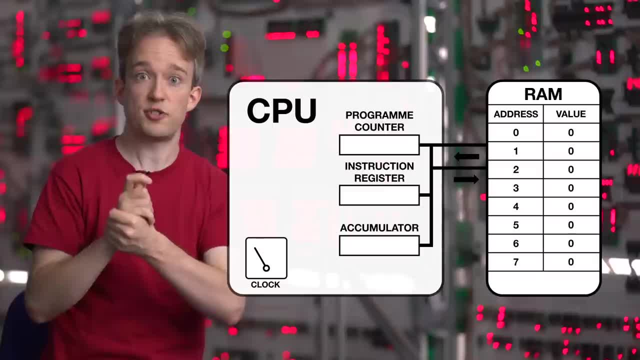 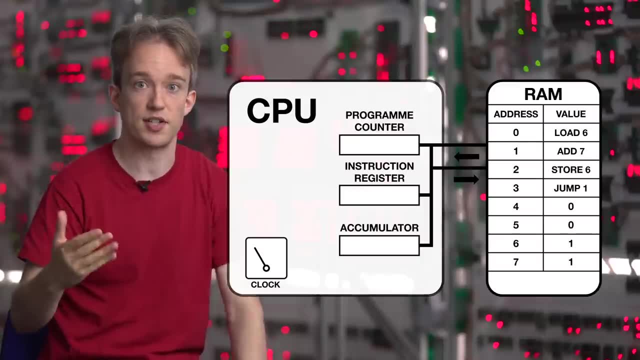 That's the one thing that's actually built into it. So we need some instructions actually in memory. So let's load our program into RAM. That RAM is also used to store our answers, our outputs In the real world. these would all be stored in binary. 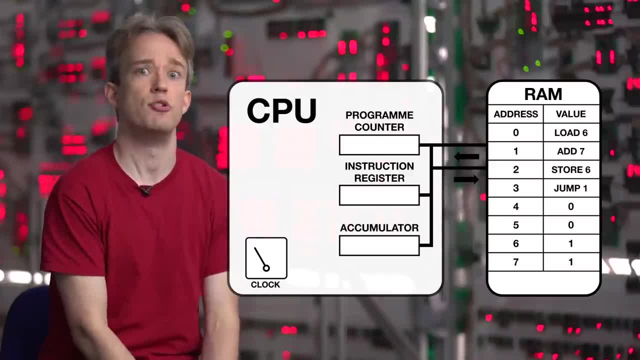 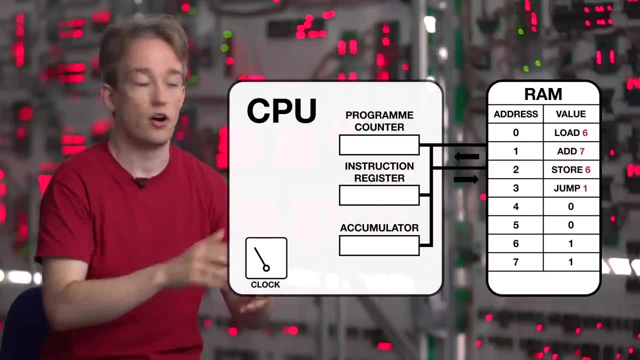 But let's not overcome that, Let's not overcomplicate things right now. let's keep them human-readable. An instruction has two parts. The first part is the instruction itself and the second part is usually a memory address. On each clock tick, the CPU will do one of three things. 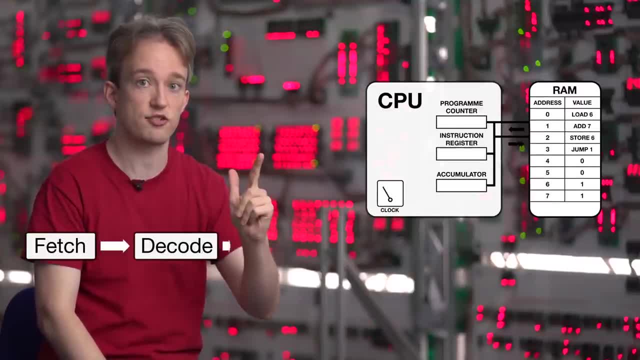 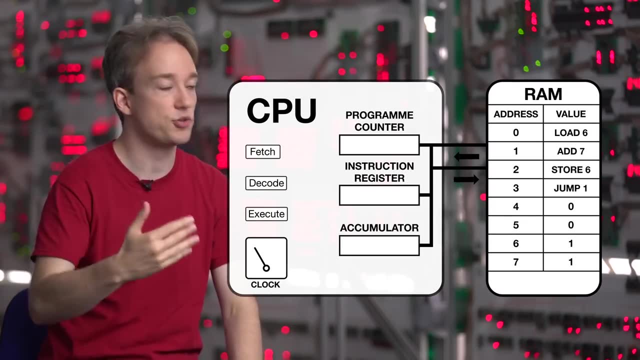 It will fetch an instruction from a memory address, It will decode that instruction and it will execute that instruction round and round in a loop. So it's going to count up, We're going to begin with a number and add one to it over and over again. 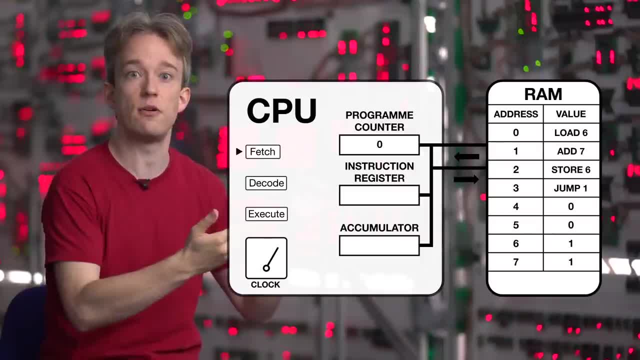 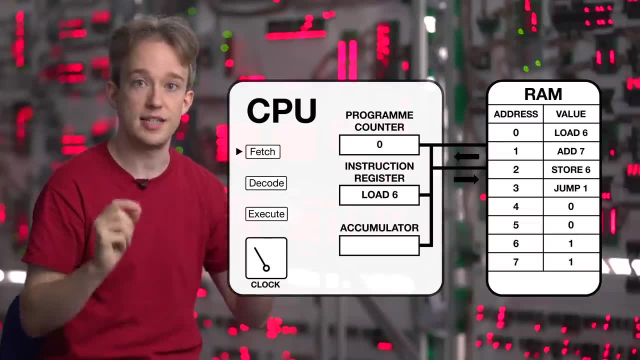 Fetch One clock tick. The program counter is set to zero. So the CPU fetches the instruction. It puts the instruction at address zero in the memory and puts it into the instruction register Decode. The CPU decodes the instruction. The first part is the instruction and the second part is a location. 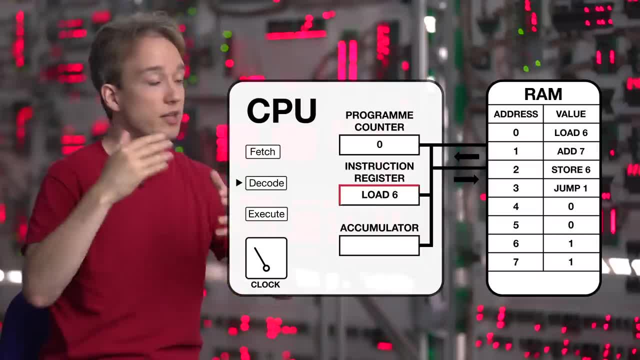 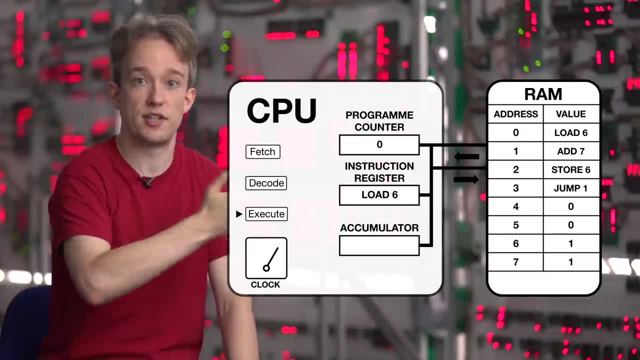 In our case, the instruction is load and the address is six, So we will be loading the value at address six into the accumulator. Execute. The CPU executes this instruction. It takes the value at address six and loads it into the accumulator. 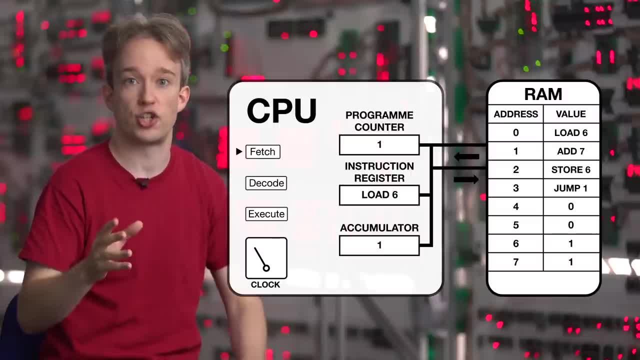 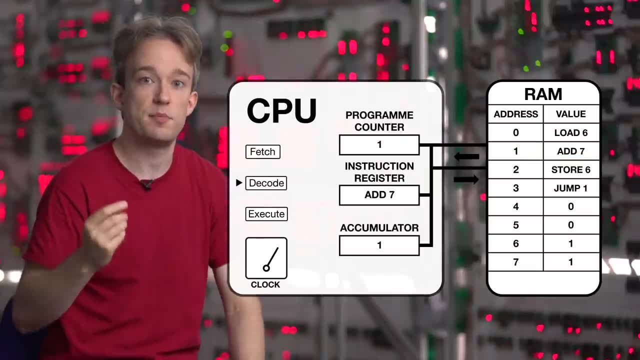 In this case the value is one. Fetch The program counter is included. It's set to zero. It's incremented. The CPU fetches the next instruction in the next bit of the memory Decode. The CPU decodes the instruction. 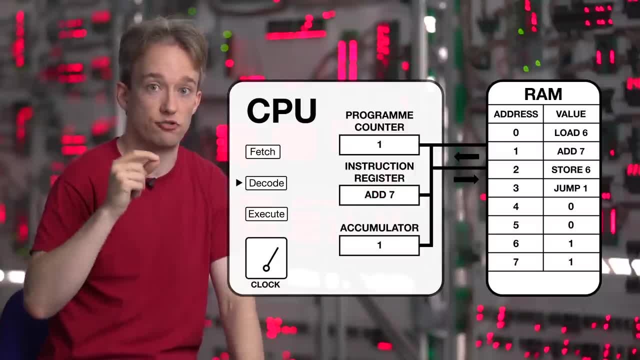 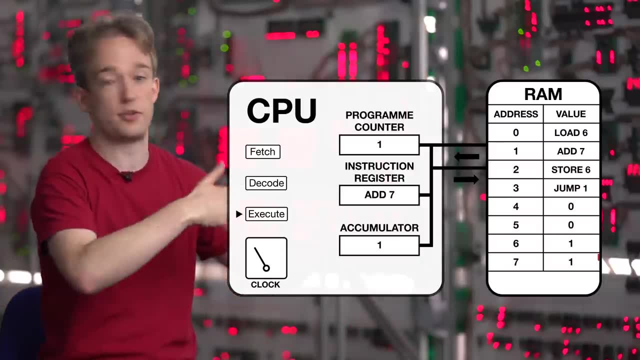 This time it's add and the address is seven. So we'll be adding what's at address seven into what is already in the accumulator Execute. The CPU executes the instruction. We add the value at address seven and in this case it's the value one. 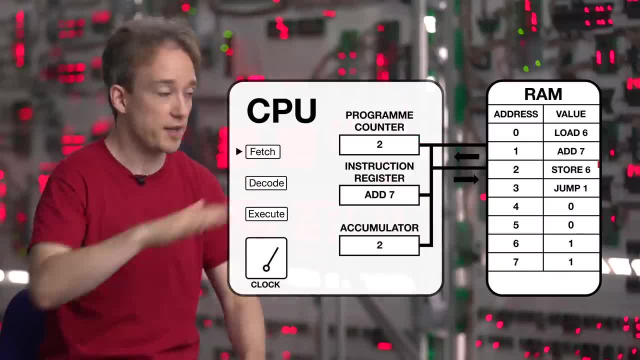 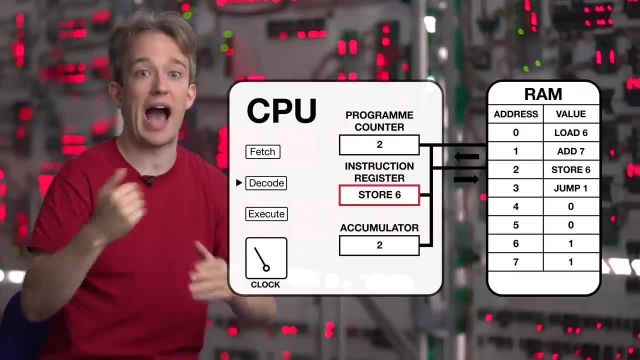 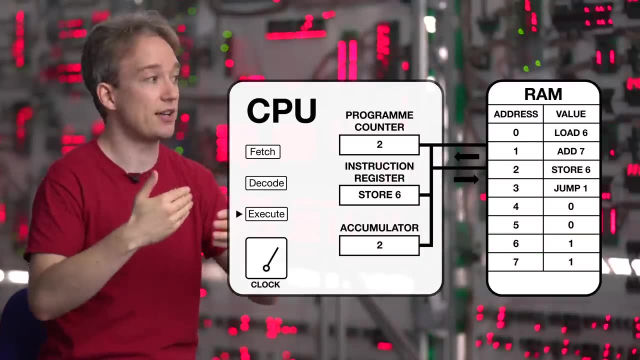 One plus one is two. Fetch From the next memory location, number two: Decode Instruction to store the value in the accumulator into RAM at address six: Execute. Now notice that we are overwriting what's already there, so address six now has two. 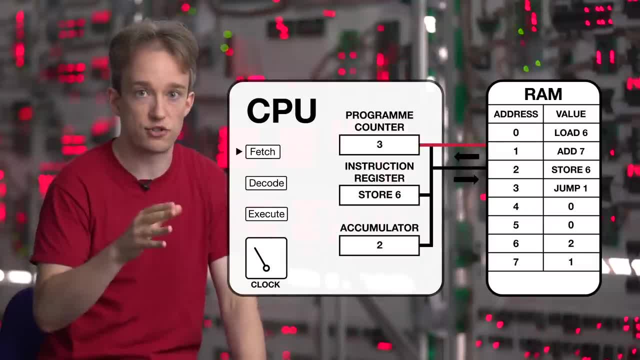 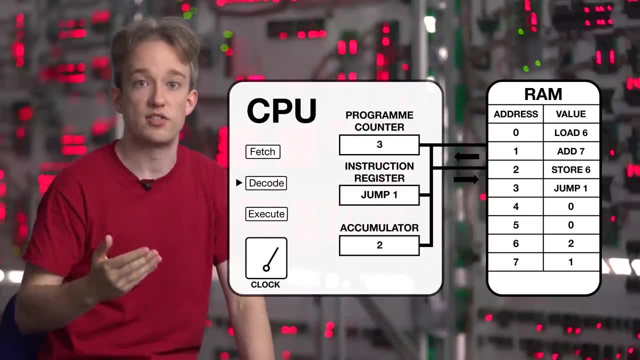 in it. instead of one, Fetch A new instruction. Jump With a jump. the next address we fetch from is the one in this instruction, Decode. So we're going to jump to address number one, Execute. The program counter is now back at one. 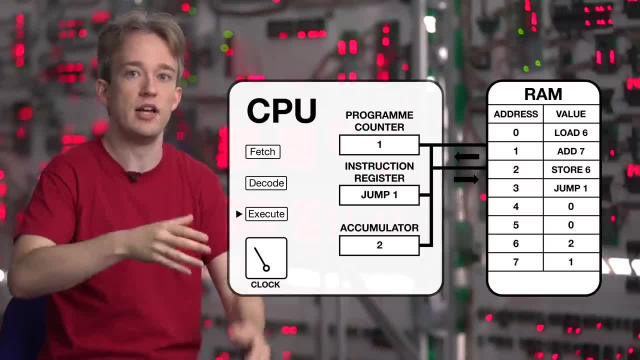 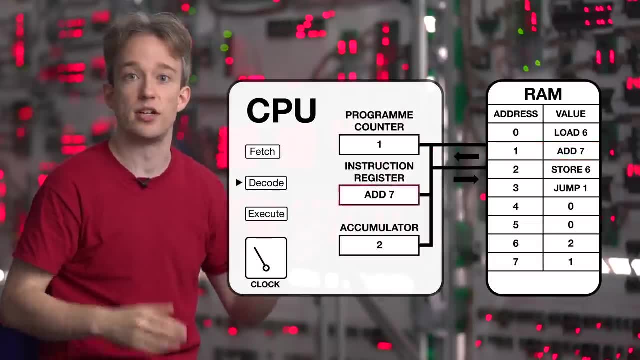 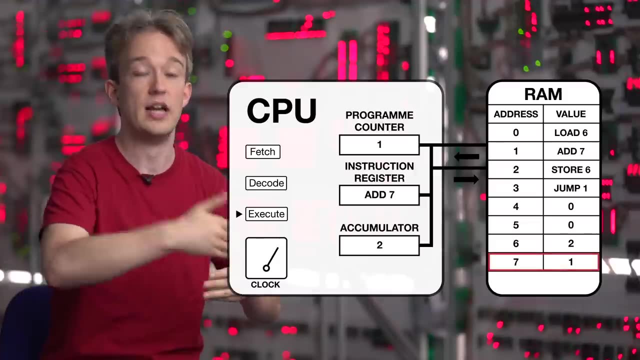 The ability to jump, To loop, To build instructions recursively is one of the foundations of computer science. So we're back up there. Fetch from location one, Decode: It's the add instruction. again Execute. Our accumulator still contains the values from before. so two plus one is three. 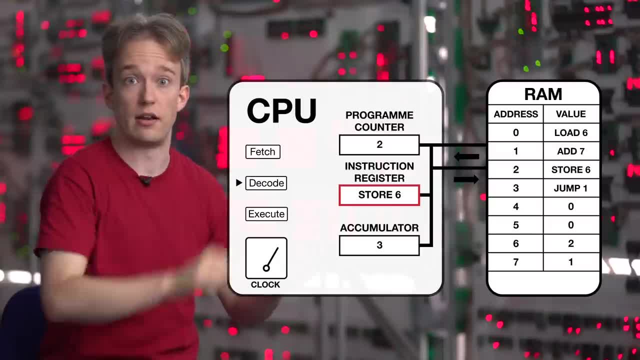 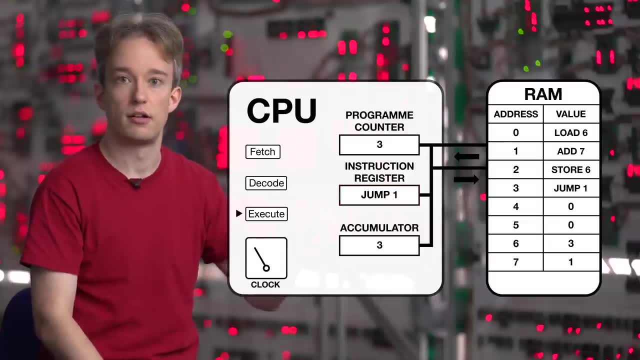 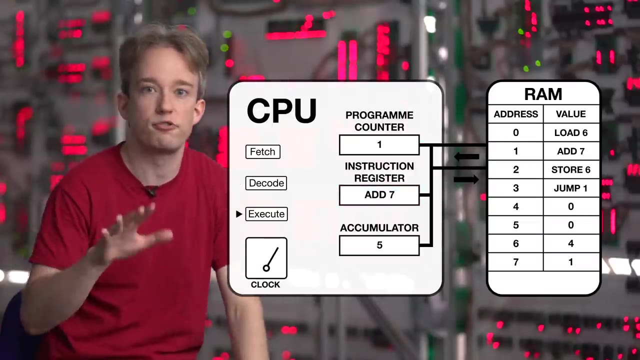 Fetch Decode- Store again Execute, Storing it into location number six. Fetch Decode- Execute. And we jump again. Fetch Decode- Execute. Fetch Decode- Execute. We're in a loop and we're counting upwards by one on every sixth clock cycle. 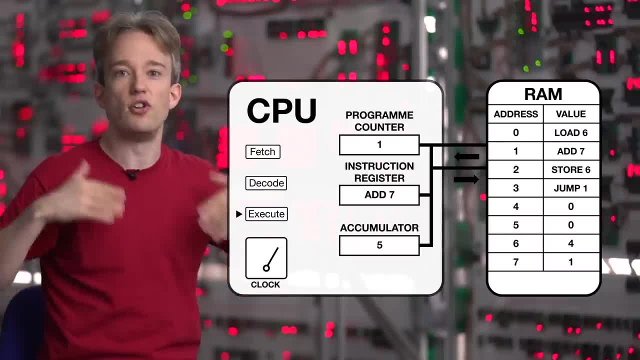 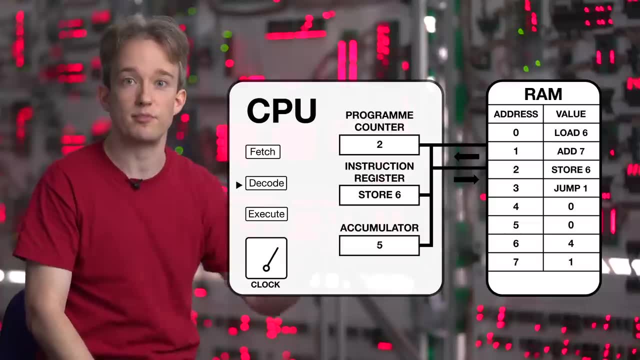 Our program with these simple instructions doesn't have a HALT command or any way to interrupt it, so it will just keep incrementing that value by one until the number becomes so large it can no longer be held by the memory address. How it breaks then. 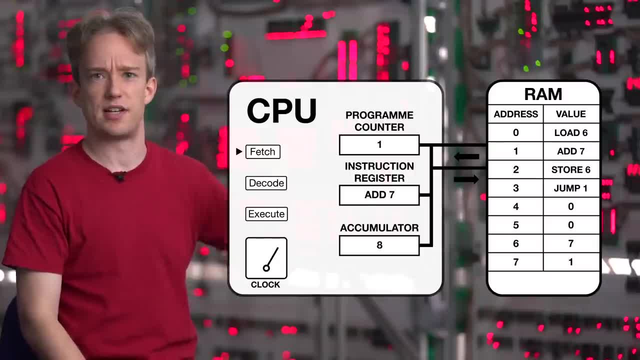 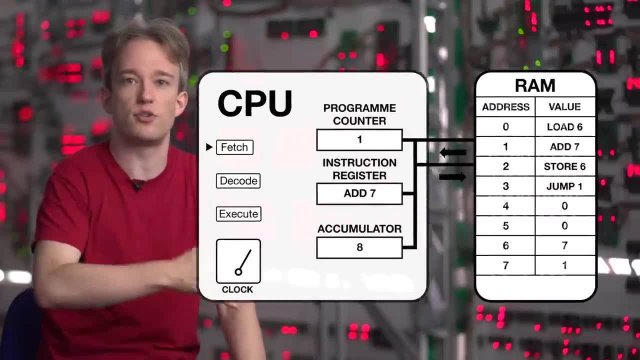 Well, that's a whole other video. Thanks for watching. My fingers are tired. This is a very fiddly way to program a computer. In theory it can be done, but at this level these instructions are just encoded in raw. 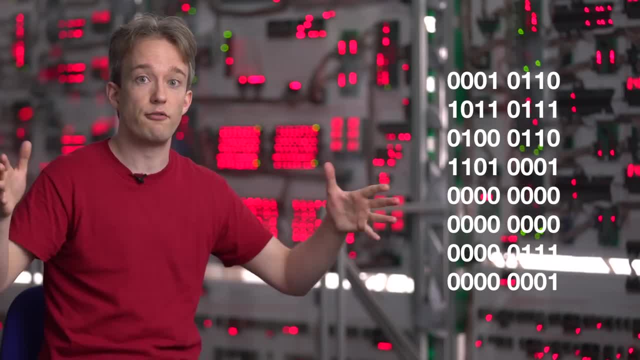 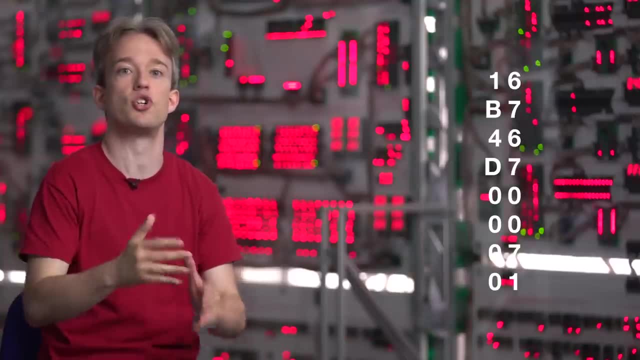 binary data which is basically unreadable for humans. So we can convert that base-2 binary to base-16, hexadecimal. At that level we call it machine code. The next step up from that is a symbolic language called assembly, which is a bit more readable. 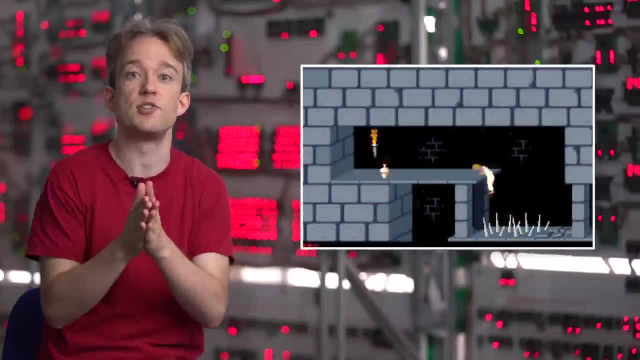 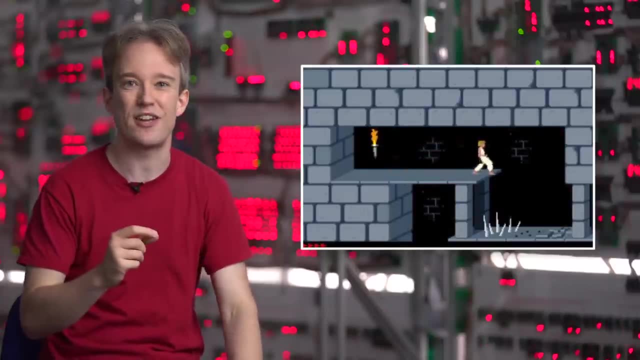 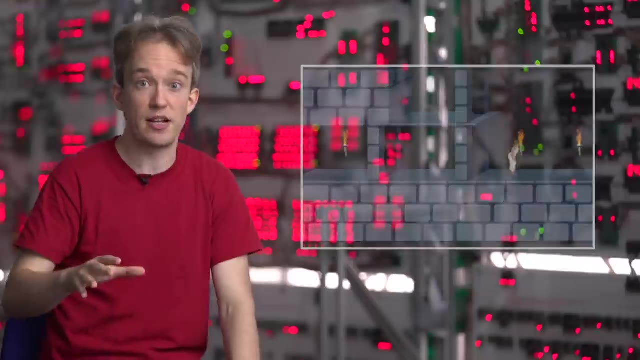 but it's still close to working at that bare metal. The original Prince of Persia game was completely programmed in assembly That is almost unbelievable: Painstakingly figuring out each pixel of animation and encoding it into something that the computer almost understands directly. 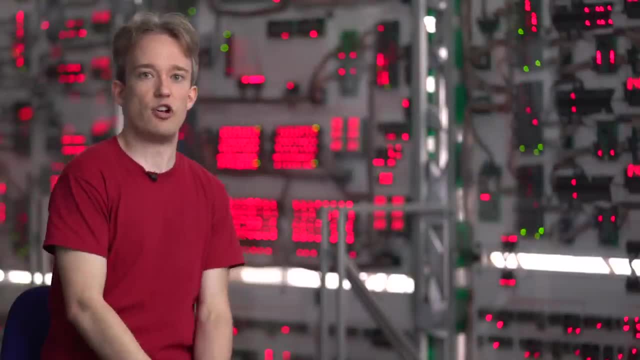 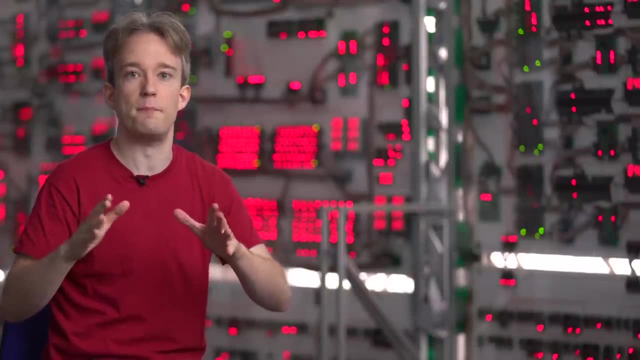 Programming like that is complex and hard and prone to the sort of human error that introduces massive security problems. It is difficult to code and difficult to debug, So, rather than dealing with the messiness or well, the pristine logic of machine code, 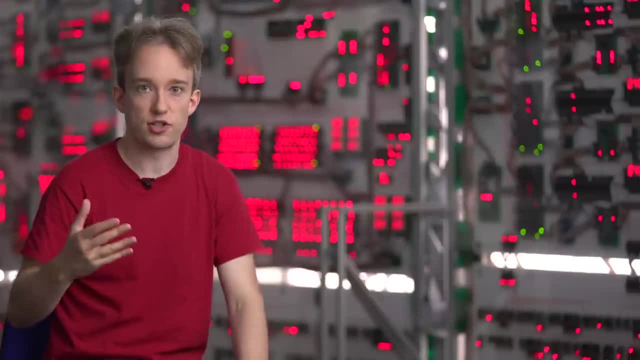 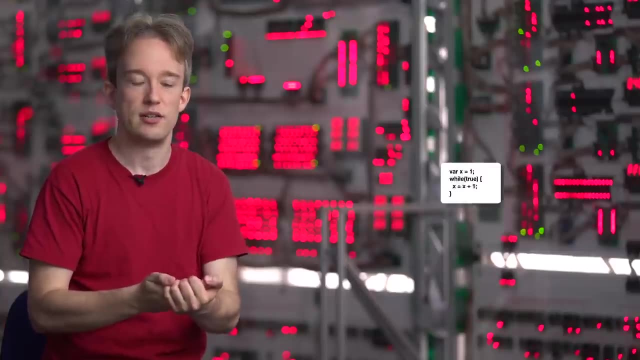 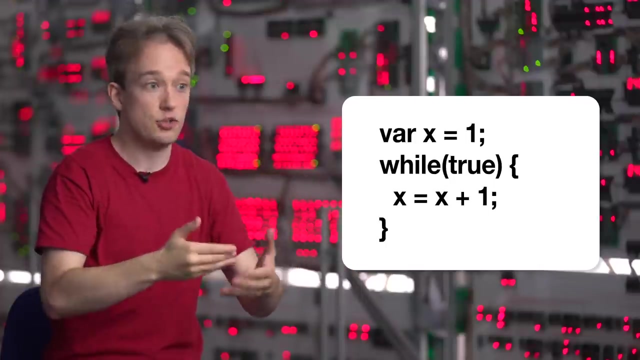 higher-level languages were developed as an intermediary step. Those languages handle all of that memory, reading and writing forward. So all we need to focus on is what we actually want the computer to do. So here's my code: Just the same instructions, phrased a little bit differently, phrased for humans to be. 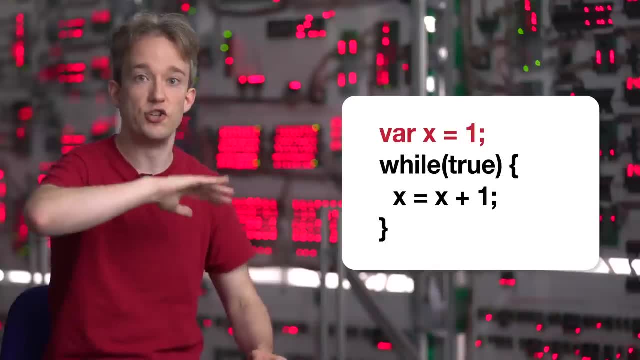 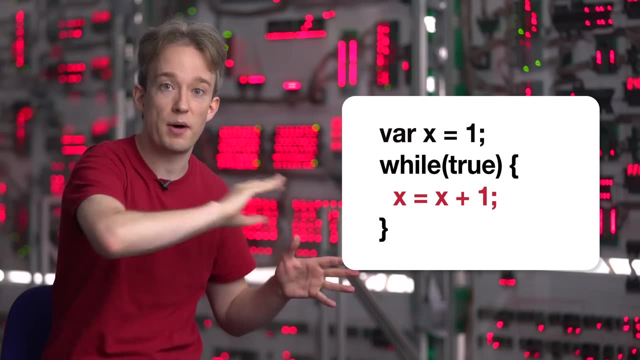 able to read. I specify a variable x. I then write a function that loops forever, and in each passing through that loop we increment x by one. Once I've written that code, I then pass it to a compiler, which turns it into that original. 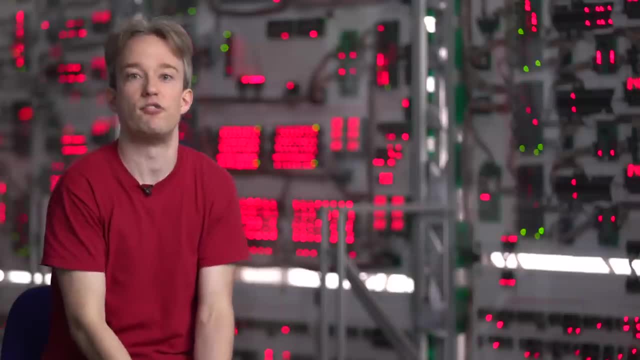 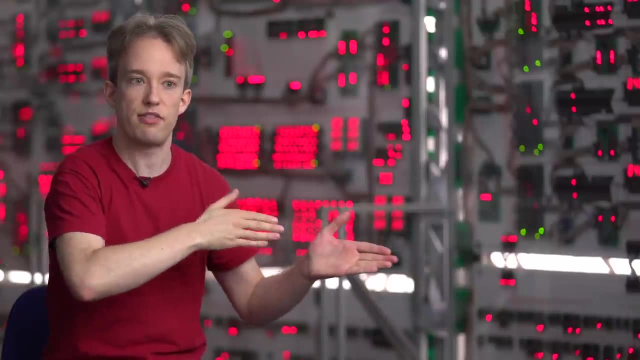 machine code for me, so when I run the program it's loaded into the computer's memory and executed. If I want to run it on a completely different type of computer- a Mac instead of a PC- I can compile it for that CPU instead. 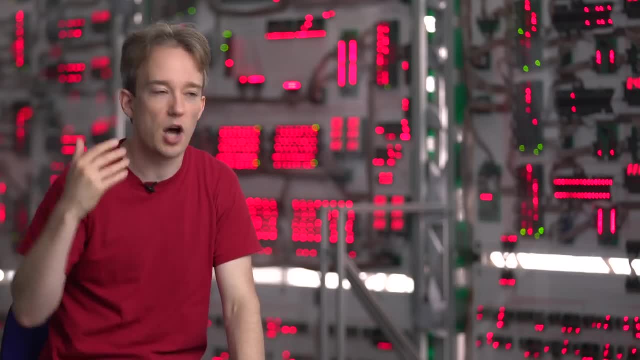 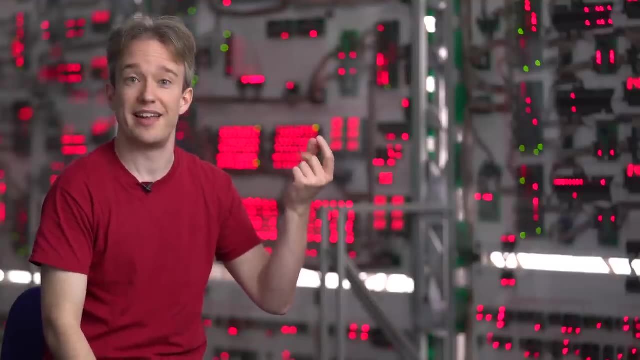 But this still doesn't answer the question of how the computer is doing something as complex as decompressing and displaying this video. The answer to that is speed. At the speed I was clicking at the end there we were executing one instruction every couple. 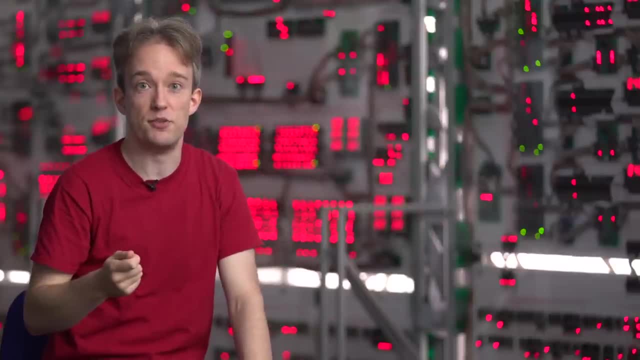 of seconds on one thread, one bit of the system. A modern CPU executes billions of instructions per second, gigahertz on multiple threads, but at the heart of your PC, on your computer, on your computer, on your computer, on your. 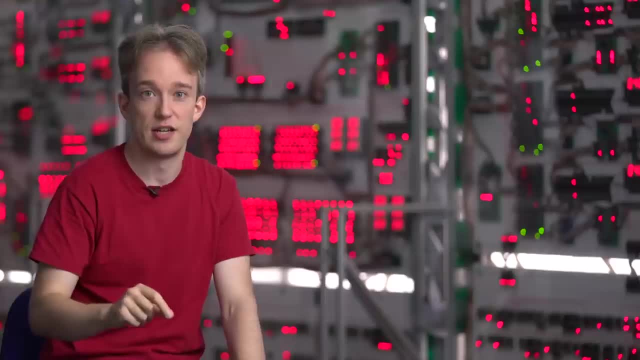 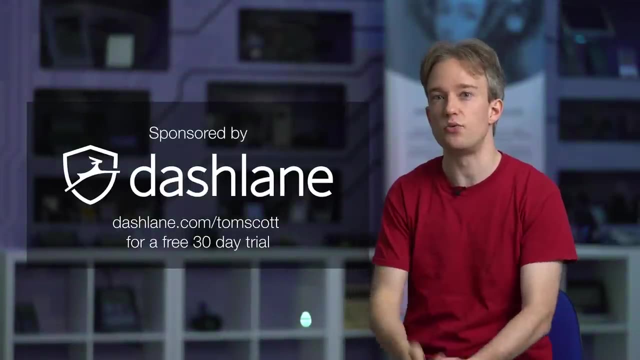 PC or your phone, there is still just a ticking clock and a fetch-execute cycle. I've used a password manager for years, and if you are techy enough to reach the end of this video, you should too- And I'm not just saying that because this video is sponsored by Dashlane. a password. 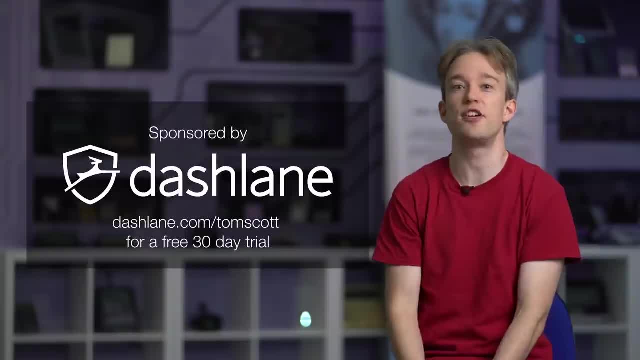 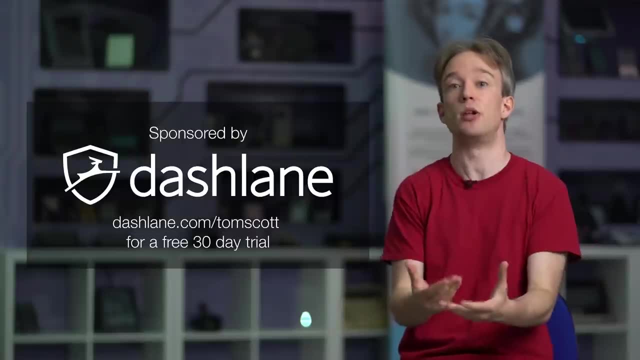 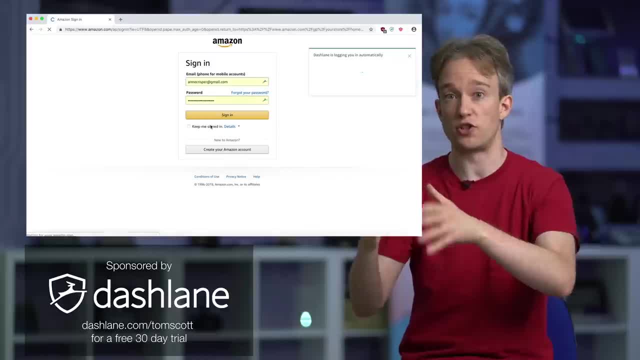 If you're like me a few years back, then you are reusing dashlanecom- slash tom scott. If you're like me a few years back, then you are reusing dashlanecom- slash tom scott. These days, Dashlane sits in my browser and when I want to log in somewhere, 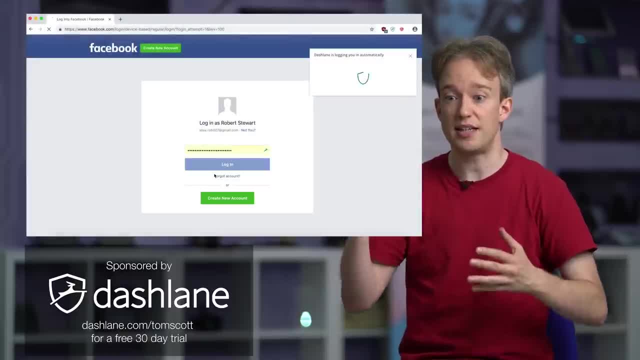 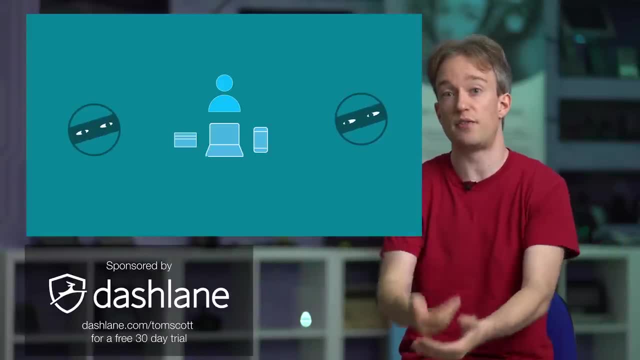 I unlock Dashlane with the single password that I have to remember and it autofills it for me. Dashlane also stores and autofills credit cards and address information across your devices and it's got a VPN to encrypt your traffic on public Wi-Fi networks, if you want to. 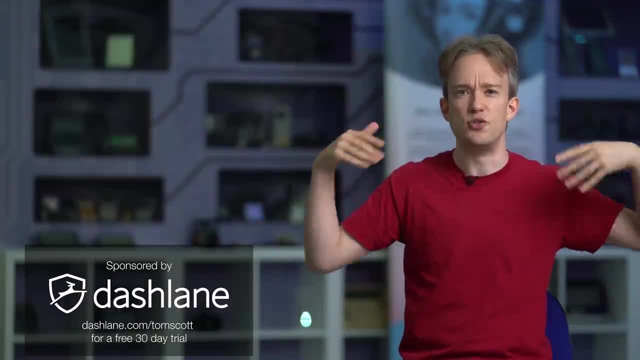 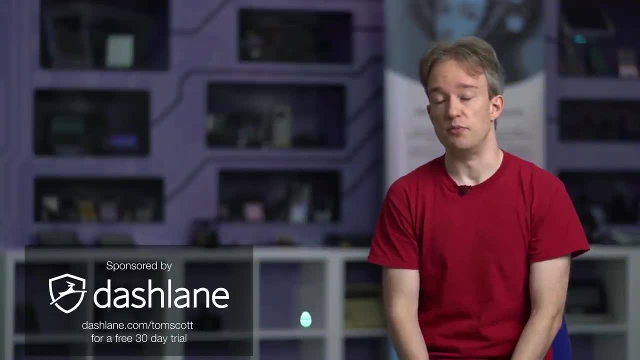 If you are the kind of person who can remember 20-character unique, symbol-filled passwords for dozens of different sites, congratulations. But if you're not superhuman, then your choice is basically using Dashlanecom. slash tom scott, Use insecure passwords or use a password manager. 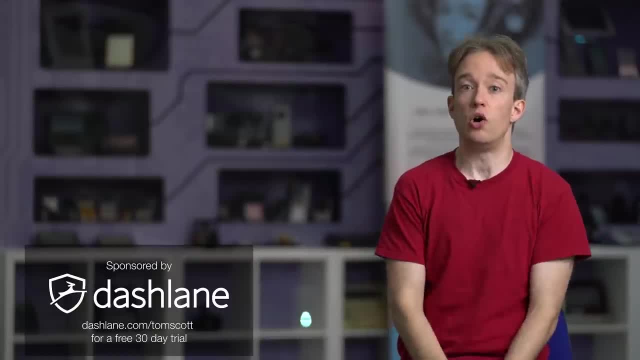 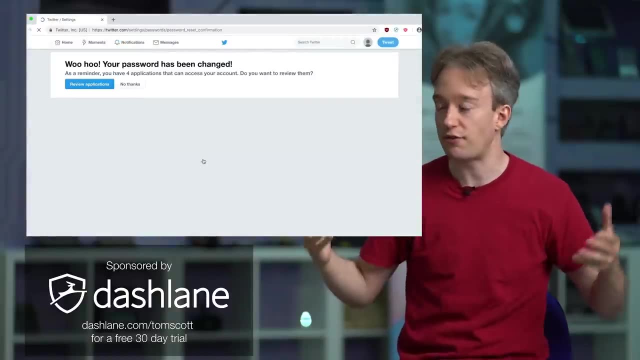 Now you could use post-it notes on your monitor as a password manager, or you could use Dashlane, which generates, stores and autofills long, secure, different passwords for every site. I don't have to try and type in a 20-character password filled with symbols on my phone anymore. 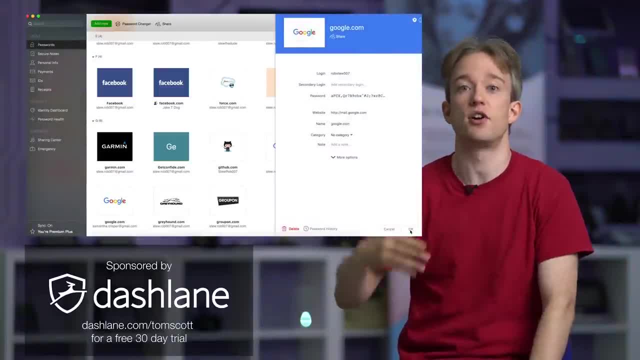 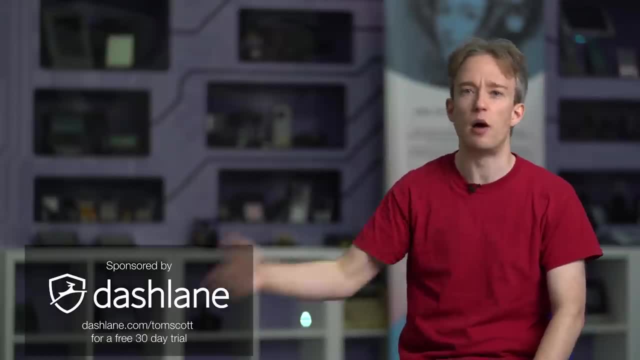 I pull up Dashlane instead. Everything just works Synchronized on all my devices across Windows, Mac, iPhone, Android, all automatically. It plugs into Chrome, Firefox, Edge, Safari, Opera. Even if you're not a computer, you can use Dashlanecom. slash tom scott.